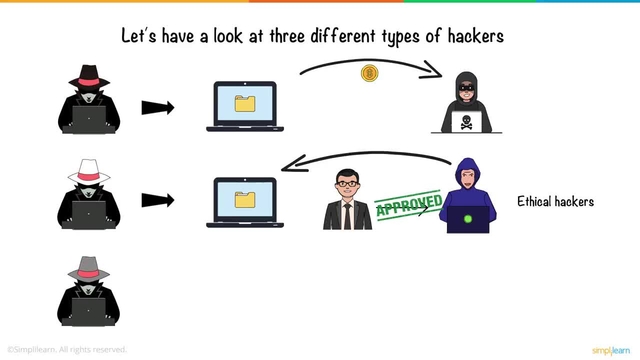 In addition to these hackers, we also have the Gray Hat hackers. As the name suggests, the color gray is a blend of both white and black. These hackers discover vulnerabilities in a system and report it to the system's owner, which is a good act. 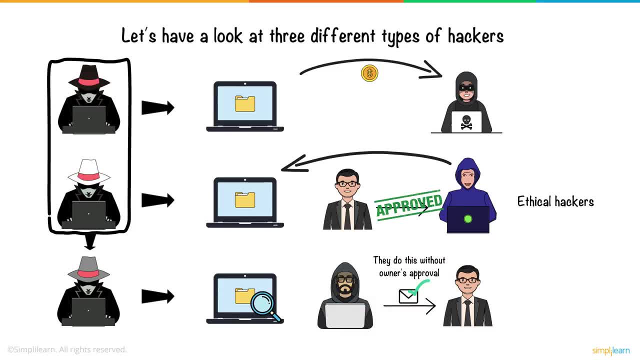 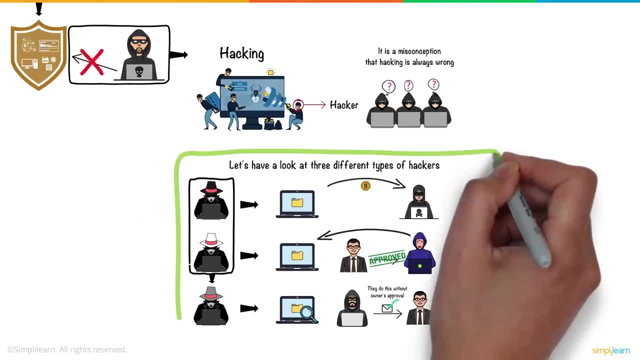 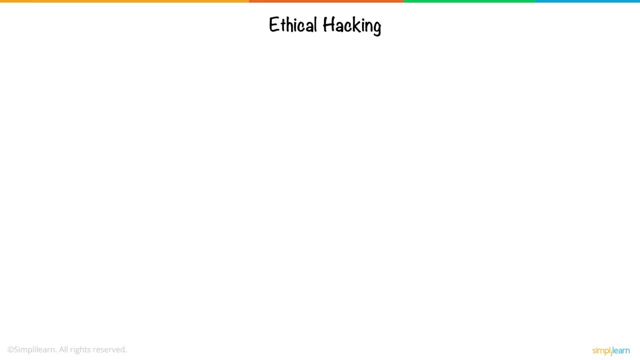 But they do this without seeking the owner's approval. Sometimes, Gray Hat hackers also ask for money in return for the spotted vulnerabilities. Now that you have seen the different types of hackers, let's understand more about the hacking that is legal and valid, ethical hacking, through an interesting story. 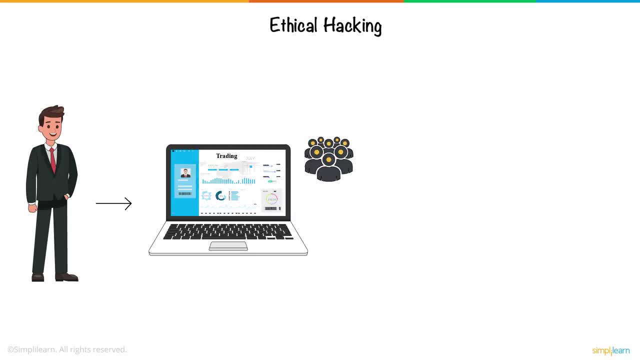 Dan runs a trading company. He does online training with the money he makes And he helps his customers invest. Everything was going well and Dan's business was booming until a hacker decided to hack the company's servers. The hacker stole the credentials of various trading accounts. 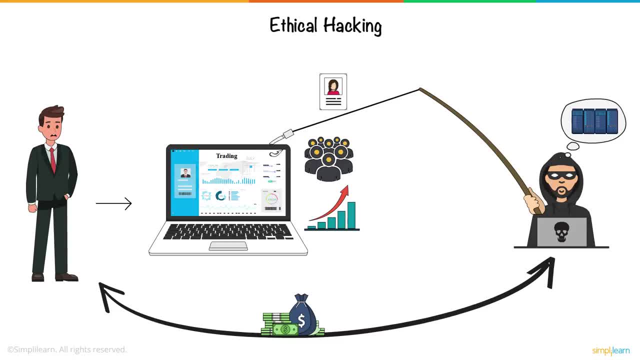 He asked for a lump sum ransom in exchange for the stolen credentials. Dan took the hacker's words lightly and didn't pay the hacker. As a result, the hacker withdrew money from various customers' accounts and Dan was liable to pay back the customers. 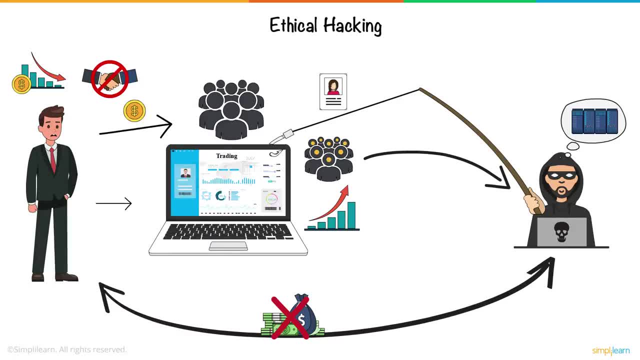 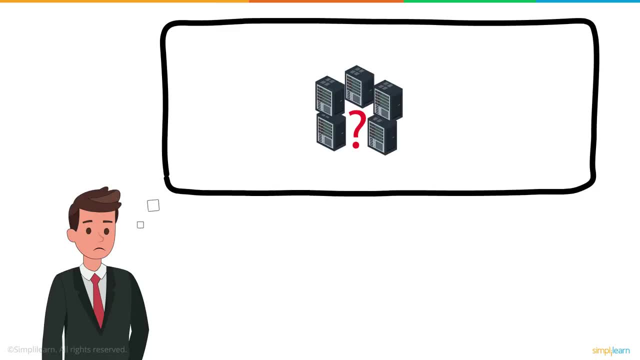 Dan lost a lot of money And also the trust of his customers. After this incident, Dan gave a lot of thought as to what could have gone wrong with the security infrastructure in his company. He wished there was someone from his company who could have run a test attack to see how vulnerable his systems were before the hacker penetrated into the network. 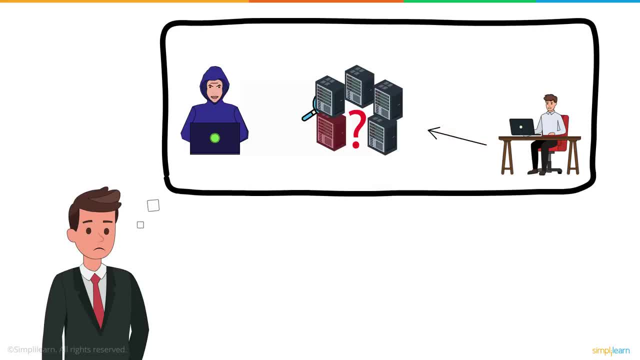 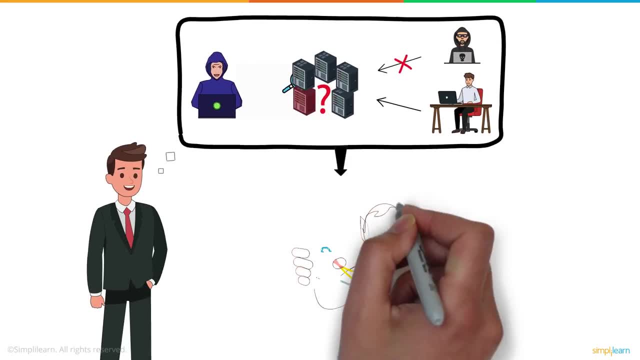 This was when he realized he needed an employee who thinks like a hacker and identifies the vulnerabilities in his network before an outsider does. To do this job, he hired an ethical hacker, John. John was a skilled professional who worked precisely like a hacker. 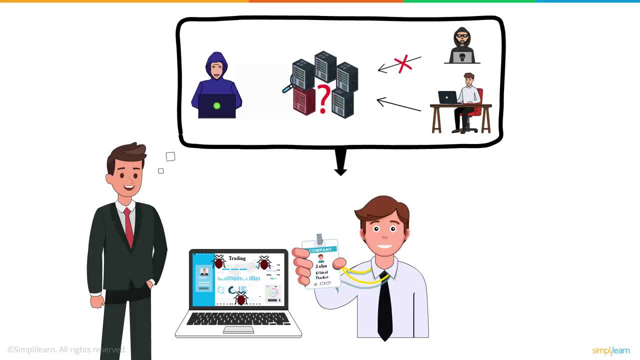 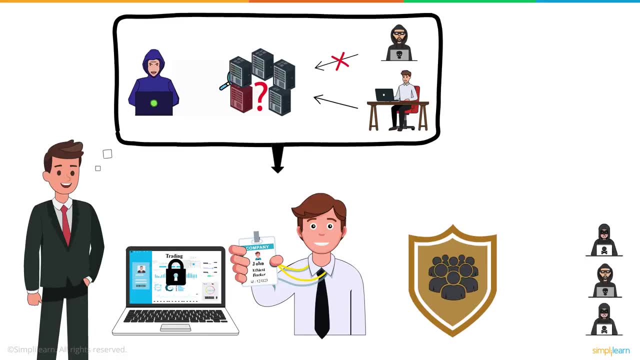 In no time. he spotted several vulnerabilities in Dan's organization and closed all the loopholes. Hiring an ethical hacker helped Dan protect his customers from further attacks in the future. This, in turn, increased the company's productivity and guarded the company's reputation. 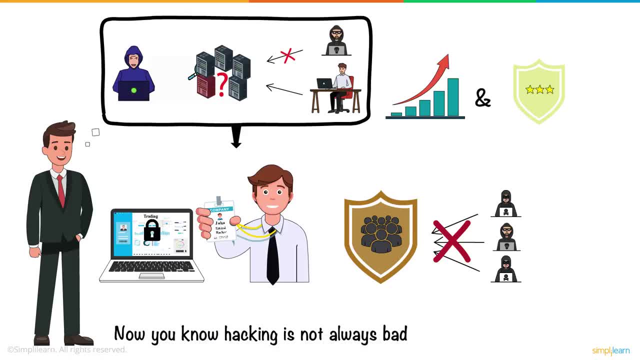 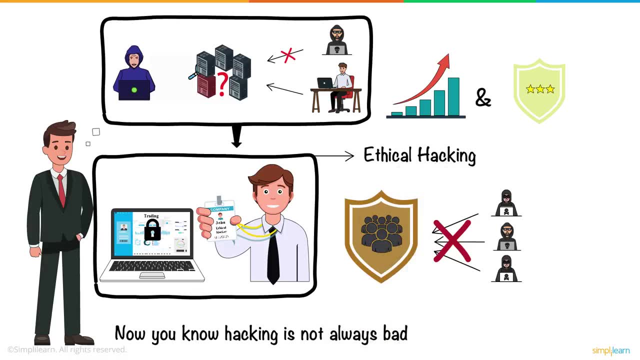 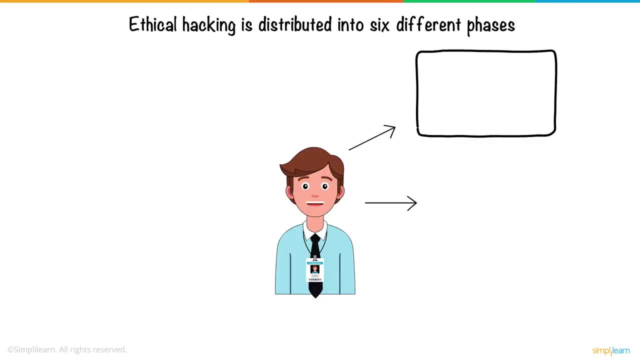 So now you know hacking is not always bad. John, in this scenario, exposed the vulnerabilities in the existing network, And such hacking is known as ethical hacking. Ethical hacking is distributed into six different phases. Let us look at these phases step by step with respect to how John, our ethical hacker, will act. 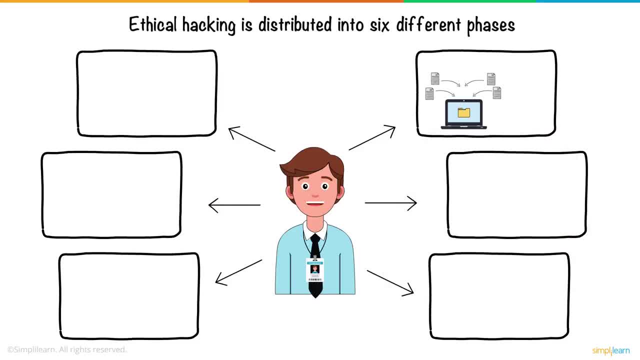 Before launching an attack, the first step John takes is to gather all the necessary information about the organization's system that he intends to attack. This step is called reconnaissance. He uses tools like Nmap and HPing for this purpose. John then tries to spot the vulnerabilities. 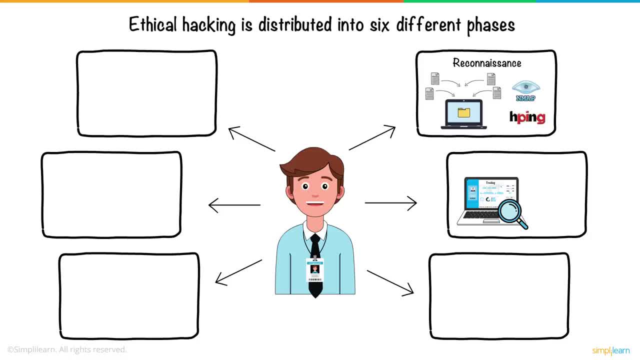 If any, in the target system using tools like Nmap and Expose. This is the scanning phase. Now that he has located the vulnerabilities, he then tries to exploit them. This step is known as gaining access. After John makes his way through the organization's networks, he tries to maintain his access for future attacks by installing backdoors in the target system. 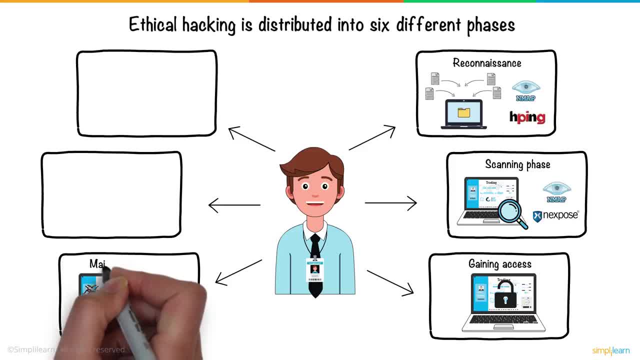 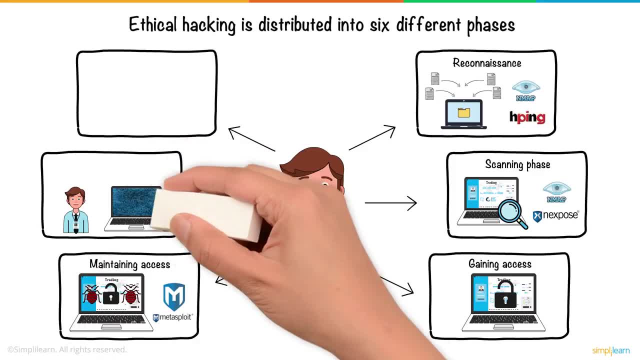 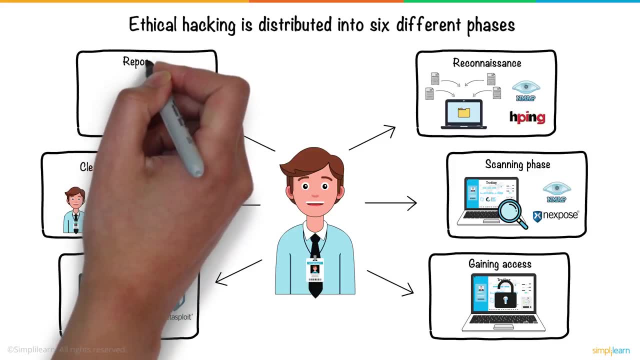 The Metasploit tool helps him with this. This phase is called maintaining access. John is a brilliant hacker, Hence he tries his best not to leave any evidence of his attack. This is the fifth phase, clearing tracks. We now have the last phase, that is, reporting. 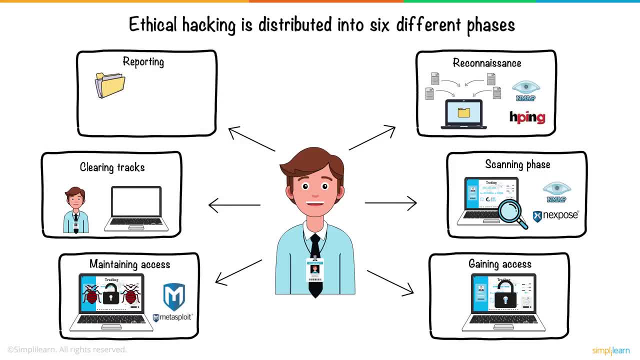 In this phase, John documents a summary of his entire attack, the vulnerabilities he spotted, the tools he used and the success rate of the attack. Looking into the report, Dan is now able to take a call And see how to protect his organization from any external cyber attacks. 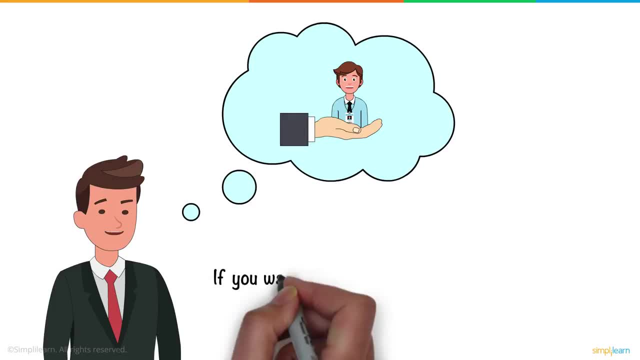 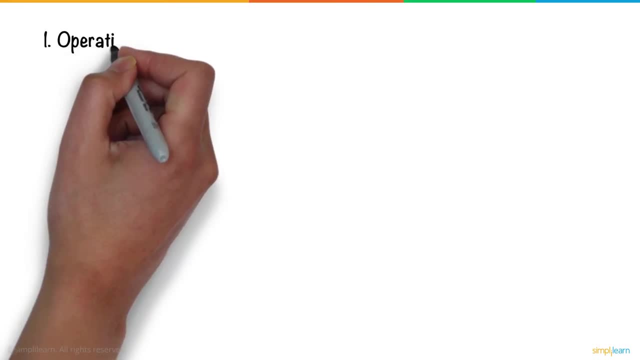 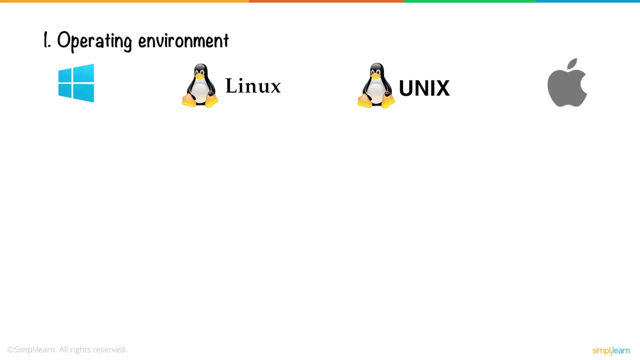 Don't you all think John is an asset to any organization? If you want to become an ethical hacker like John, then there are a few skills that you need to acquire. First and foremost, you need to have a good knowledge of operating environments such as Windows, Linux, Unix and Macintosh. 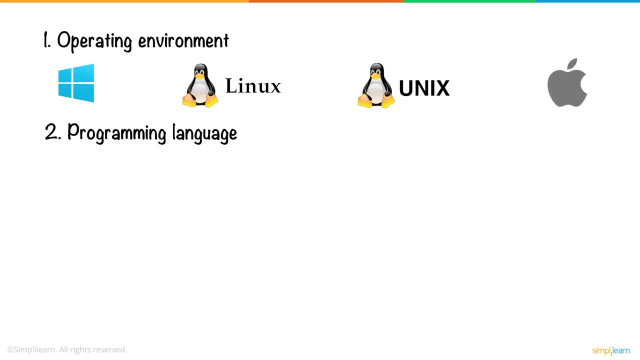 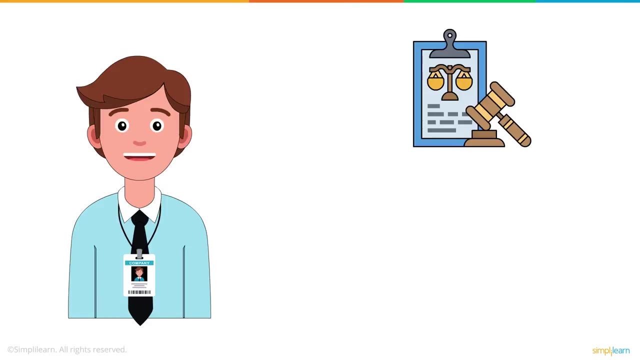 You must have reasonably good knowledge of programming languages such as HTML, PHP, Python, SQL and JavaScript. Networking is the base of ethical hacking, Hence you should be good at it. Ethical hackers should be well aware of security laws so that they don't misuse their skills. 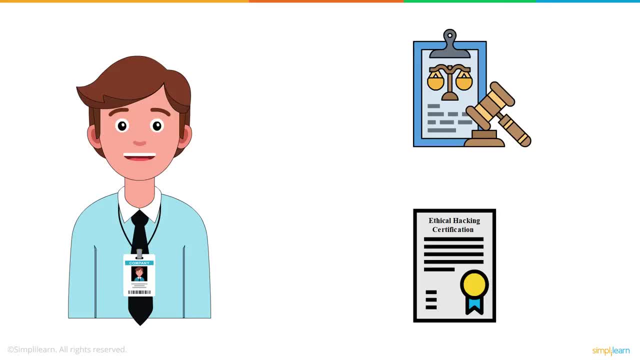 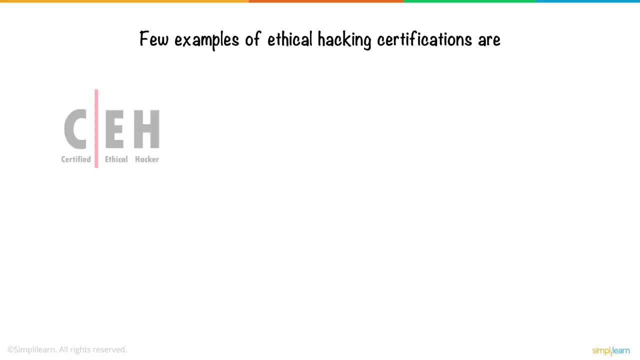 Finally, you must have a global certification on ethical hacking to successfully bag a position of an ethical hacker like John Few. examples of ethical hacking certification are Certified Ethical Hacker Certification, CompTIA, PenTest Plus and Licensed Penetration Tester Certification, to name a few.